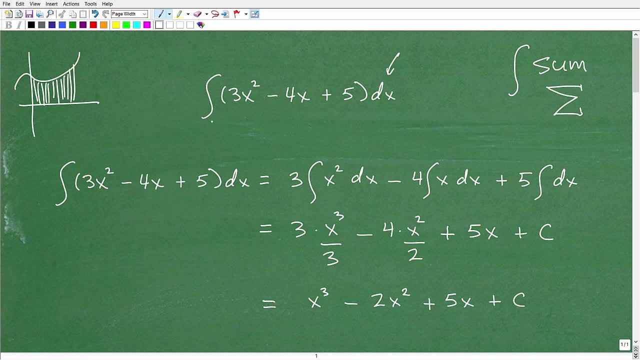 upper and or lower and upper limits. So maybe, like, say, three to seven, we would be finding the area underneath the curve from three to seven. Now, we're not going to be do do. we're not going to do that in this particular problem. All we're trying to do is just find the anti-derivative or just find the integral of this particular function. All right, So, as my titles stated, this is a basic problem for those of you out there are learning this, Of course: finding the integral. 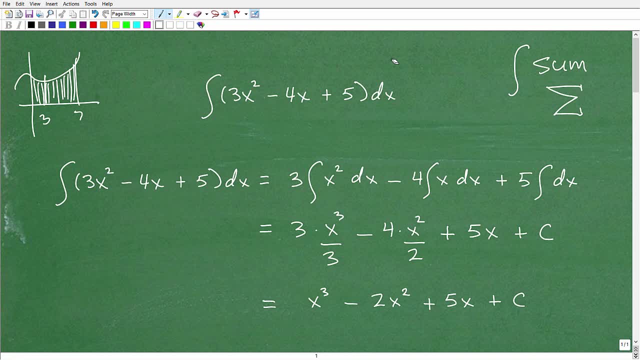 there. First of all, there's many, many, many rules. Okay, Doesn't get, this can get quite challenging. So, wherever you are, wherever you are at in calculus, just know that calculus has tons and tons and tons of rules that you know you're going to have to kind of memorize or simply just have good notes. And if you look in any calculus book, there's all kinds of cheat sheets and formulas. So you want to, you know, obviously have those at your ready, But you got to, of course, know how to employ. 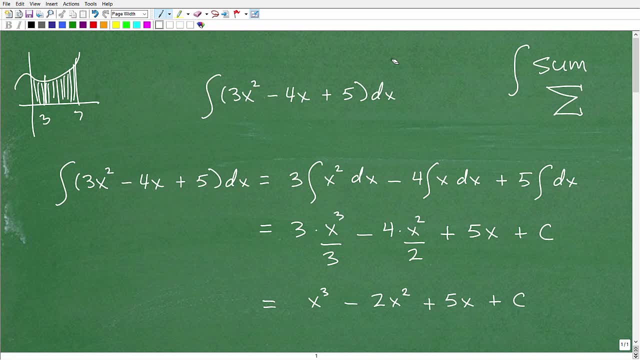 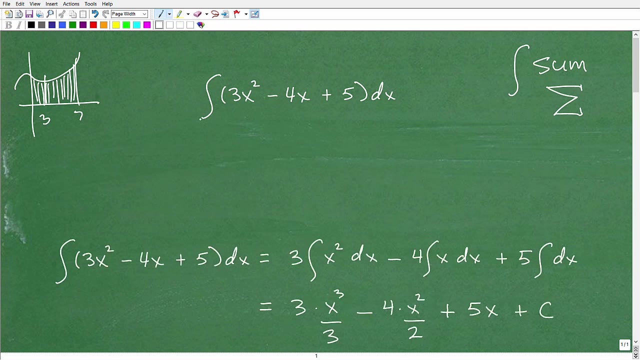 those formulas and rules. So let's go ahead and take a look at this problem and kind of illustrate some basic concepts of the integral. Okay, We're finding the integral, All right, So we're going to find the integral of this function. Now, one of the main things you can do in calculus and go ahead and give myself some room here is: we're finding the integral of this entire function. What I can do is just find the integral of each individual term. So I could just say: okay, I'm going to find the integral of three x squared, Okay, Minus. 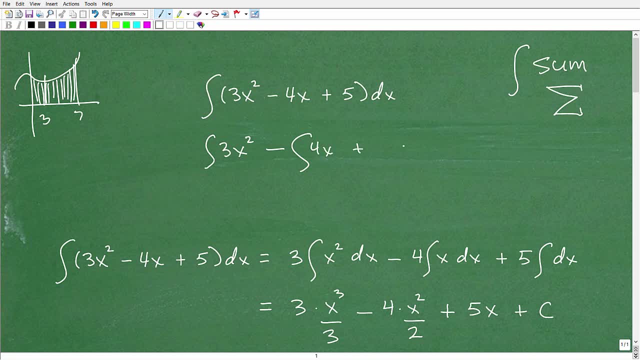 the integral of four, x plus integral of five. Okay, So, first thing is, I can break up my integration into its individual components with these terms. All right, So that's a fundamental principle of integration, a rule that you need to know. Okay, And it's going to come in handy. Probably I can be using this rule all the time when you're doing integration problems, Okay. 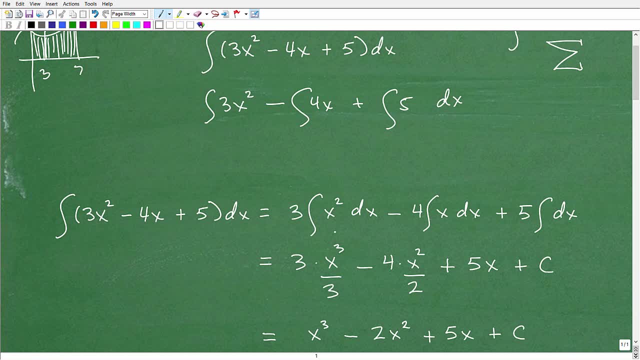 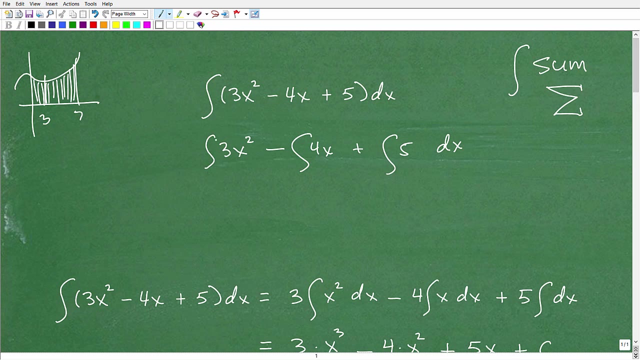 So the next rule- and of course I have this kind of broken out down here a little bit more thoroughly, But let's go ahead and just talk about the next rule before you see this here- is we can factor out the constants in this particular problem. So, for example, the integral of three x squared. I could factor out this constant. So it's going to be three times the integral of x squared minus. here I could do the same thing. 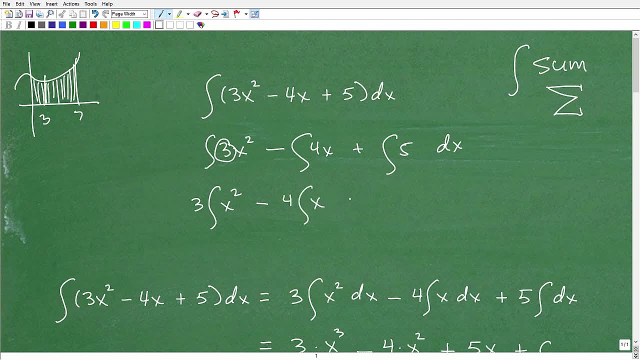 Four times integral of x plus here This is just going to be the integral of five dx. Okay, So that's the next major kind of principle here that you can do in terms of integration. Again, this is the real basic, fundamental concepts of integration, Some of the initial rules that you learn. Okay, So hopefully this is pretty easy for you Now if you. 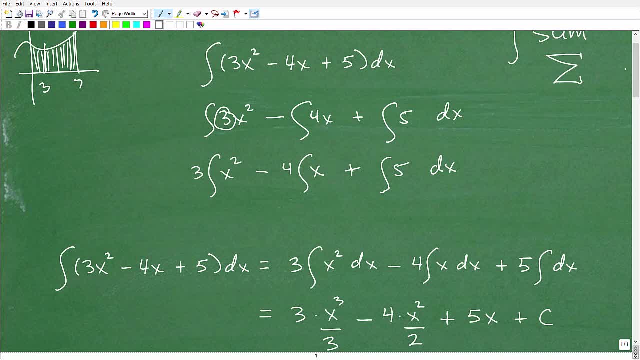 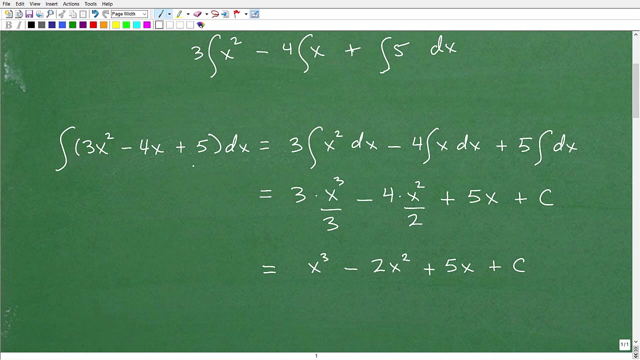 those you out there watching this problem and didn't know this. and you are taking calculus, you know, don't beat yourself up, but just you know, you know, be mindful that these are kind of, you know, the introductory type of concepts of integration that you kind of need to learn And they're, you know, used all the time. All right, So now, with that being said, let's go ahead and take a look at our problem. So we started off with this integral problem, So you can see how I can write it like. so Okay, And, by the way, technically here, 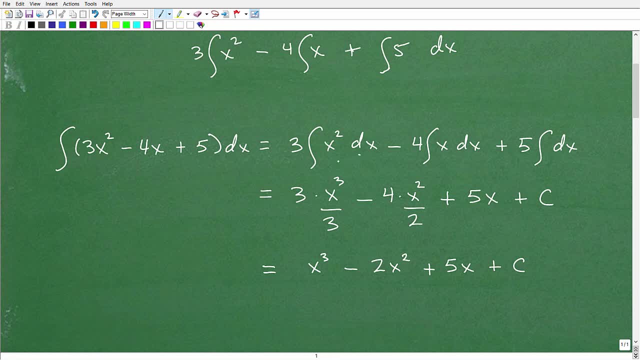 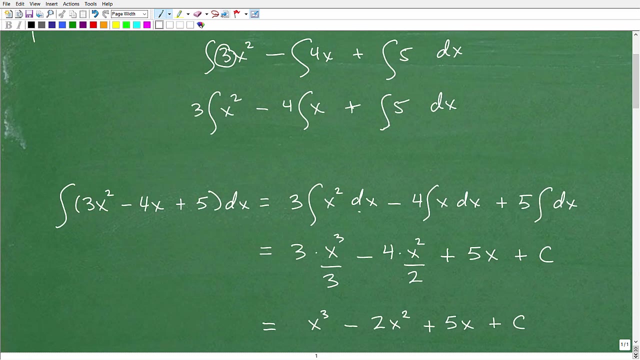 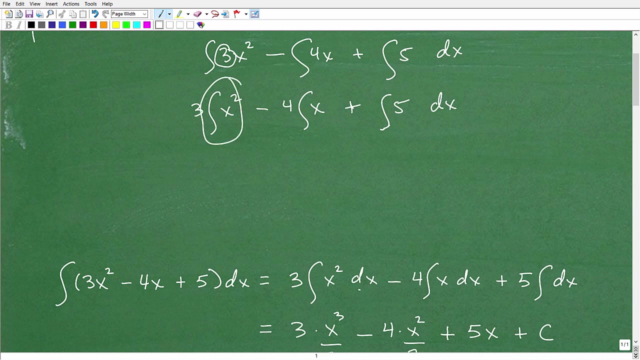 that's most correct to write the little dx after each one, because we are. these are kind of three separate integration problems, So you don't want to put your little dx behind each one of these terms. Now, at this point, let's go ahead and take a look at the actual integration. Okay, like- and this is where it gets interesting- So let's take a look at this part of the problem. Okay, Well, let's just actually look at this whole thing right here. 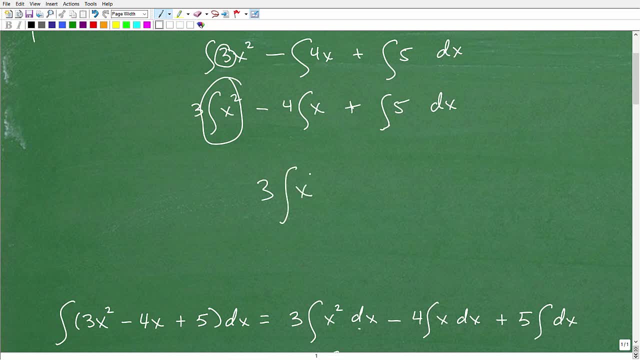 So three integral of x square. All right, So now we want to find the anti derivative, we want to get rid of this elongated s and actually evaluate the integral. So how do we do that? Well, again, you're going to have to know many, many, many rules. Okay, One of the most basic rules that comes in handy all the time is the power rule. Okay, And there's different ways of kind of showing you that theorem of integration. 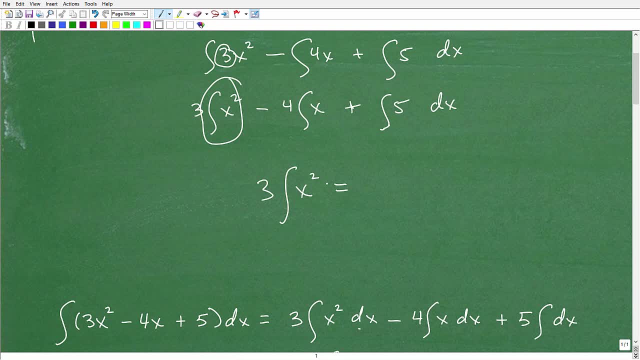 I'm definitely not trying to give you a technical lecture here, But I do want to kind of explain it. So here, if you have a function, okay with a variable to some power, like so what you can do is this: x squared. here let's just actually look at this problem a little bit more isolated. integral of x squared is equal to the, this variable x. Okay, what we do? we take this power, we add one to it, So it's going to be two plus one. we leave that in the exponent And then we're going to go ahead and do that. 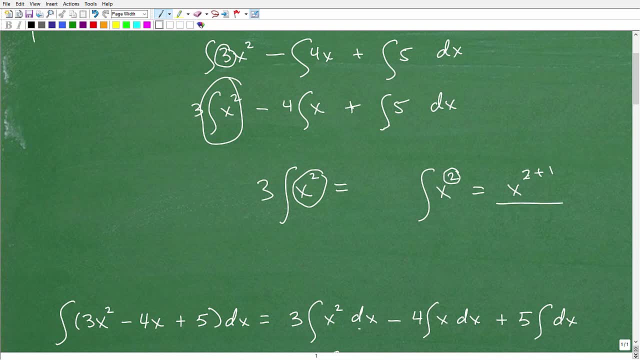 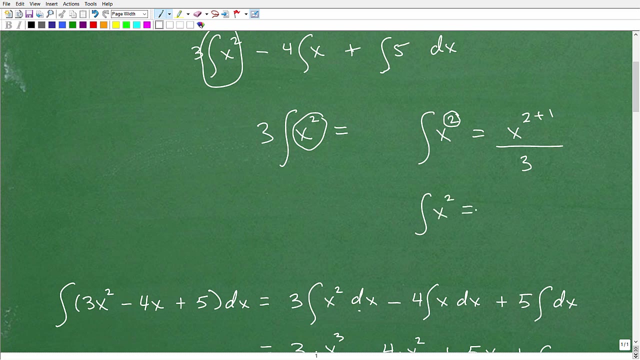 ahead and divide this term by this sum 2 plus 1, which of course is 3. okay, so the integral. go ahead and write this down here: integral of x squared is equal to x cubed over 3. okay, all right, that is what we call the power rule. all right, but there's different ways to describe it, different theorems. 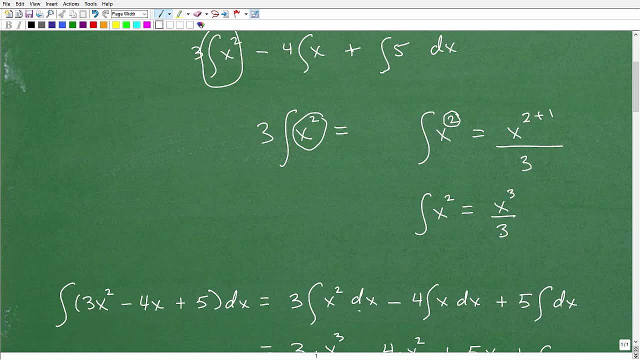 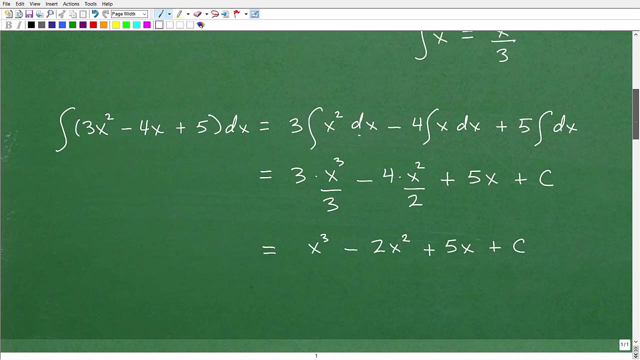 etc. but this is one key principle of integration. now there's all kinds of different rules that you're going to need to know about integration, so you don't want to confuse them, but we obviously we want to master the basic rules. so, knowing that, okay, we can come back here and take a look at our 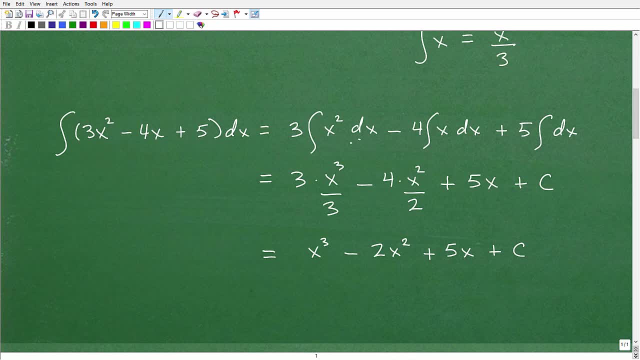 problem. so we start off with our, our integral problem, and we broke it up, okay, into its individual terms, broke up at this. we broke this up into three integration terms, all right, and we factored out the constant. so here we can see our x squared. we took the integral, so this is going to be three times. 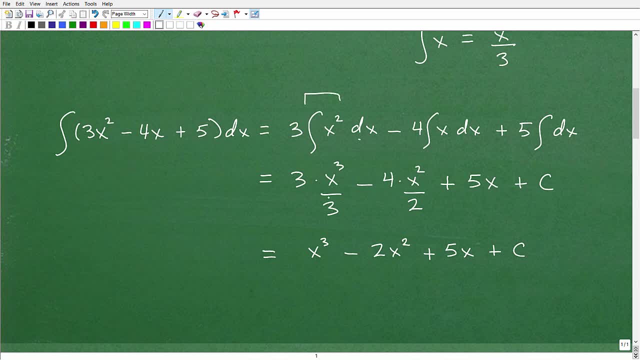 the integral of x squared, which is x cubed over 3, as i just described. okay, the dx goes away and here you can see each one right. so here this is going to be four times the integral of x, which is going to be what? x? i'm going to add one to it, so it's going to be x to the first, so it's going. 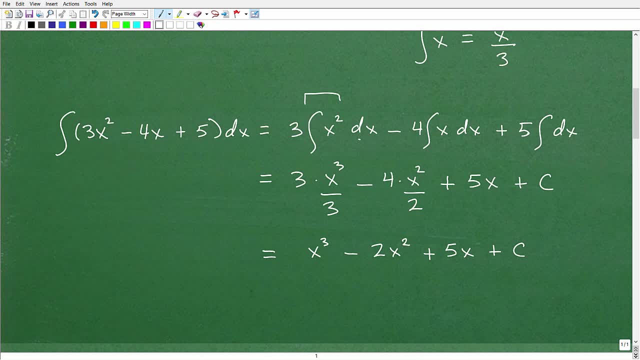 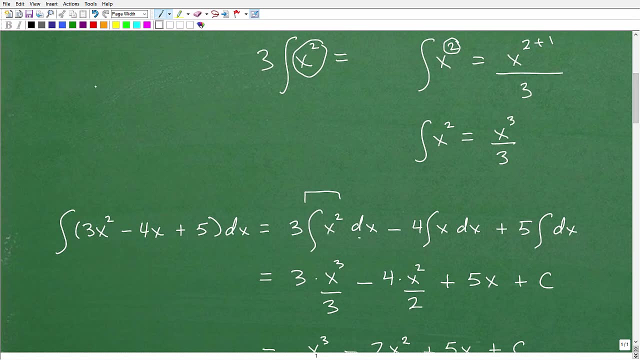 to be x squared over two, and then this five. okay, um, really, what's going on here? yeah, technically speaking, the integral of five, this is x to the zero power, okay, which is just one. so that's why we're going up by one, okay, x to the first divided. 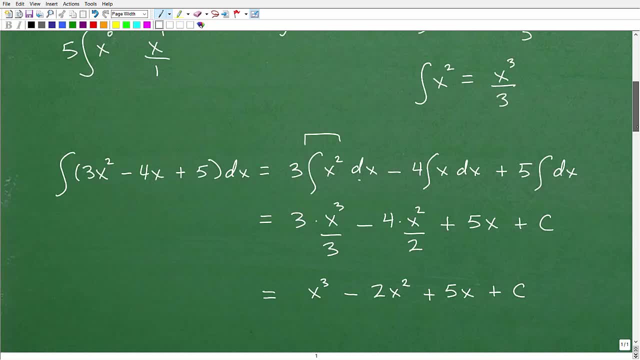 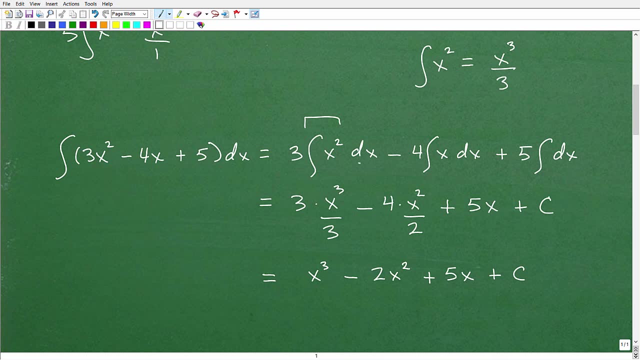 by one. that gives us a 5x. and then, of course, we have to add in our constant. okay, so anytime you're finding the integral of a function, you got to always put that plus c, which represents some constant. we don't know what that is, so you're going to have to always put that plus c, which is: 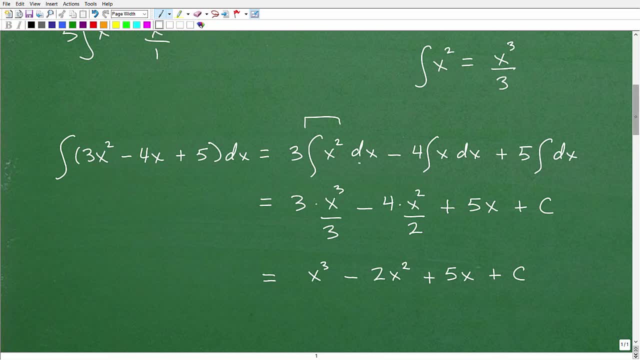 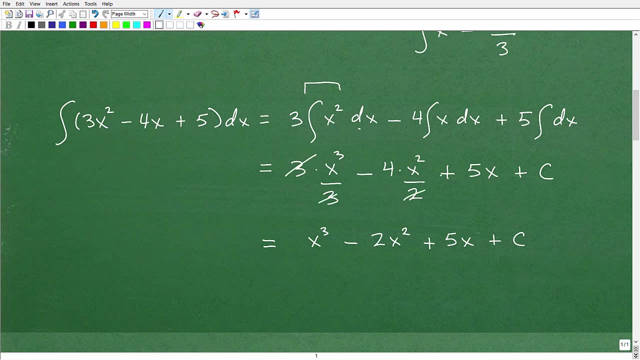 just represented as plus c. okay, so for this point four, we go ahead and just uh, employ our basic algebra skills. we cross, cancel the threes, two goes into this four, two, and then we have our 5x plus c. so this would be the integral of this, uh, basic integration problem. now, of course, if we were 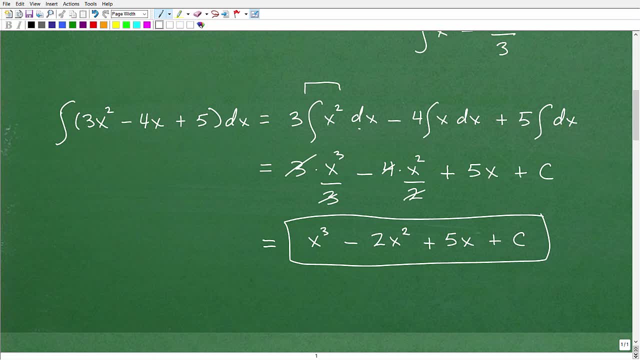 trying to find the area underneath, uh, this particular function, and it was bounded. let's say three, two, eight. then we would take this guy here and we would evaluate it from three to eight, which is a whole another uh topic in and of itself okay, but we can't find the area underneath a particular. 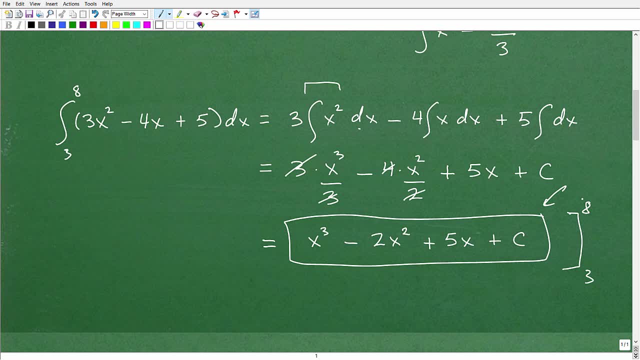 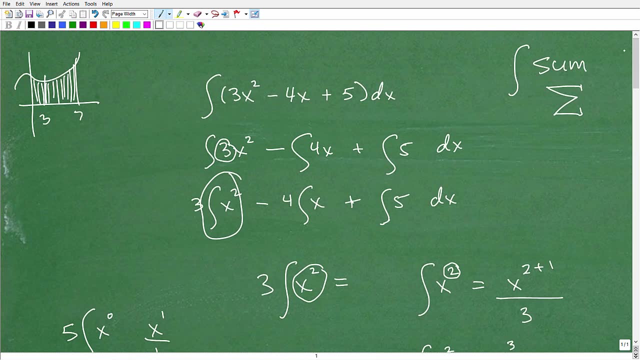 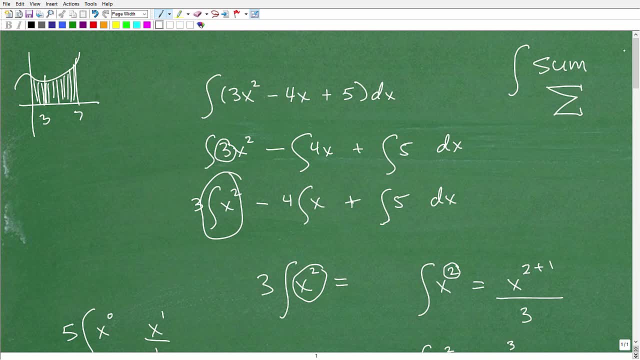 topic okay between the concepts of what uh, derivatives are, integrals are, etc. so my best advice to you is this: uh doesn't make a difference. you know how strong you are in math. the first time you take calculus it is kind of mind-boggling because it's a. there's different.